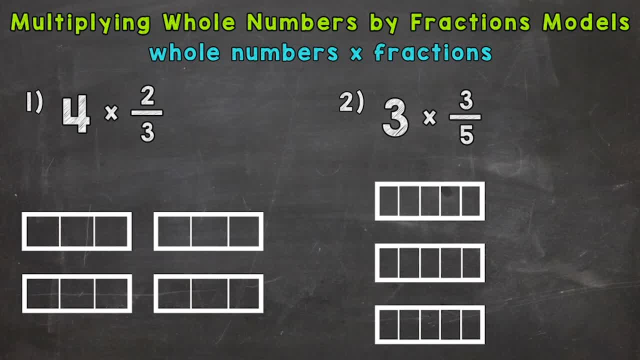 I have another video in which we do models of fractions by fractions. I'll drop that link down in the description. So let's jump into number one here, where we have four times two-thirds, So four groups of two-thirds, And, as you can notice below the problem here we have four rectangles and they're each cut into thirds. 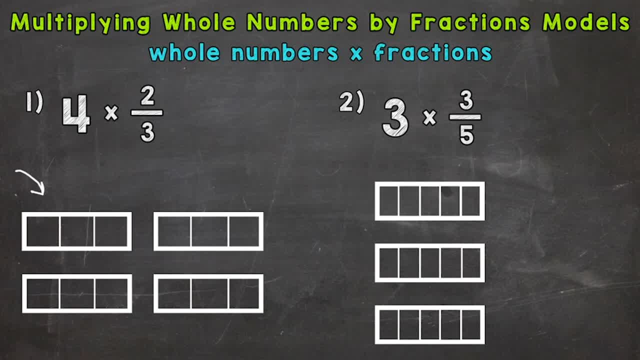 So let's create four groups of two-thirds. So here, if I fill in one, there I have one-third. If I fill in two, I have two-thirds. So that's one group of two-thirds. So that would represent one times two-thirds. 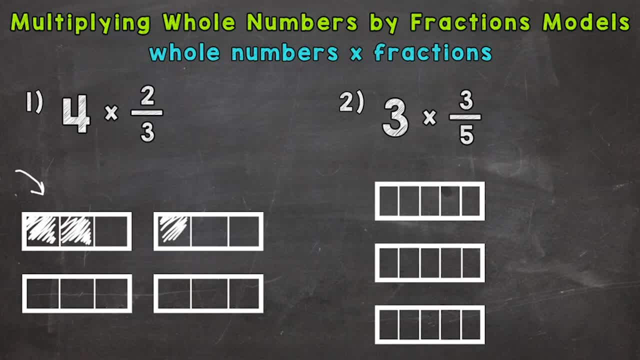 So let's do another one. There's one-third and two-thirds, So that would represent two groups of two-thirds, which would be two times two-thirds. But we want four, So let's do two more One-third, two-thirds. 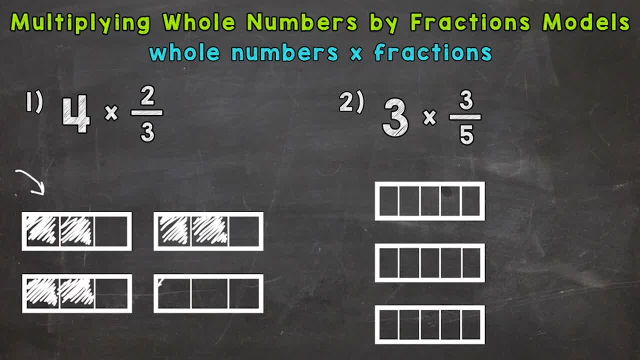 So there's one more two-thirds, And let's do the last one here. One-third, two-thirds, So we have four, Four groups of two-thirds there. Now let's see how many total thirds are filled in. So we have one, two, three, four, five, six, seven, eight-thirds filled in. 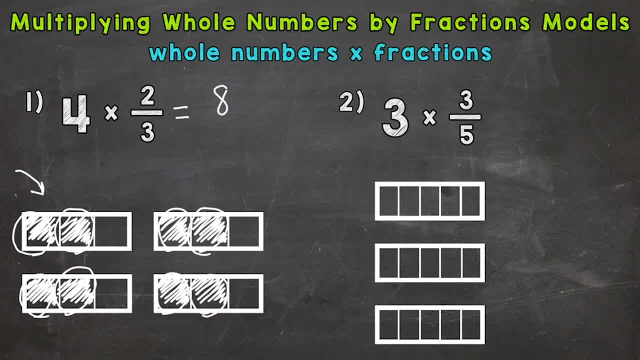 So that's going to be our numerator eight And our denominator everything's cut into thirds, so that's going to be our denominator three. That's our answer, eight-thirds. but it's an improper fraction, So let's convert it to a mixed number here. 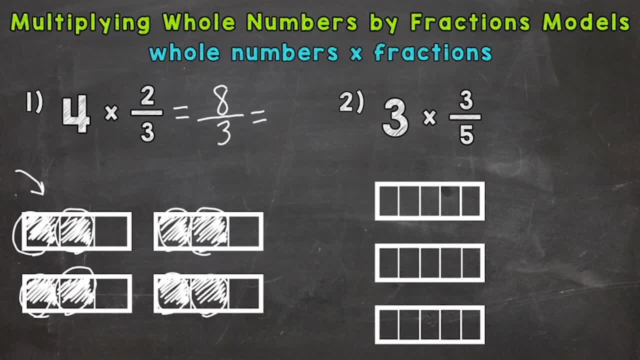 So we do that by dividing eight by three. How many whole groups of three can we pull out of eight? Well, two, That gets us to six, right, So we have a remainder. So if we pull two whole groups of three out of eight, we have two left over. 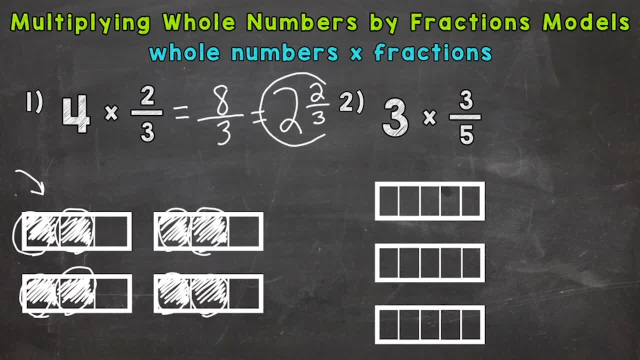 Keep our denominator the same and we get two and two-thirds. Now another way of thinking of this, or seeing that we have two and two-thirds: we could take the groups of one-thirds and kind of fill them in to make holes. 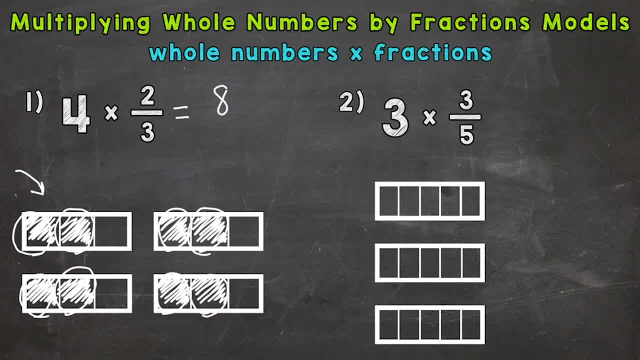 So that's going to be our numerator eight And our denominator everything's cut into thirds, so that's going to be our denominator three. That's our answer, eight-thirds. but it's an improper fraction, So let's convert it to a mixed number here. 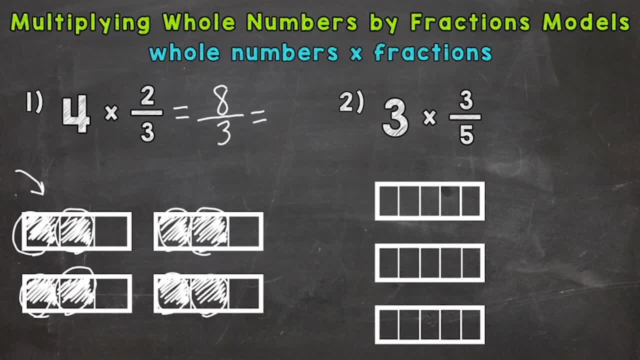 So we do that by dividing eight by three. How many whole groups of three can we pull out of eight? Well, two, That gets us to six, right, So we have a remainder. So if we pull two whole groups of three out of eight, we have two left over. 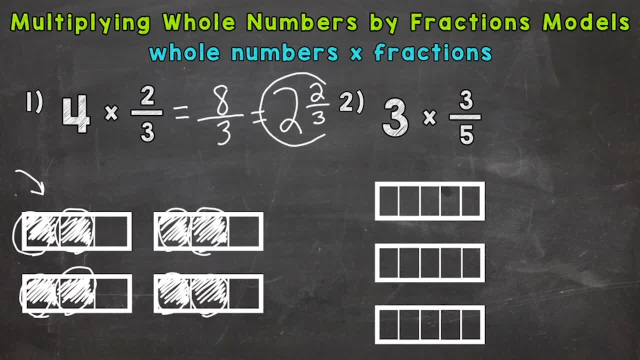 Keep our denominator the same and we get two and two-thirds. Now another way of thinking of this, or seeing that we have two and two-thirds: we could take the groups of one-thirds and kind of fill them in to make holes. 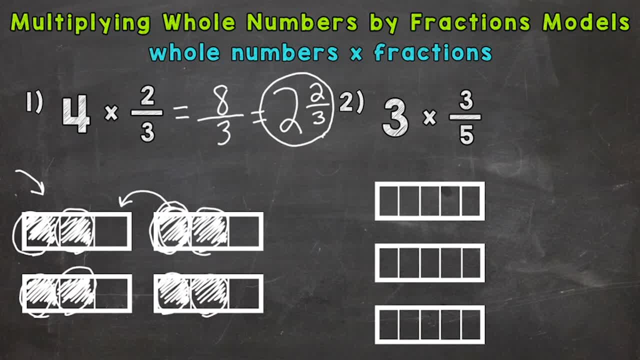 So that would make one hole there. if we filled that in, That would give us two openings: This one and right there. since we moved it, Let's move this to an opening and this to an opening, And that would give us Two holes filled in, right. 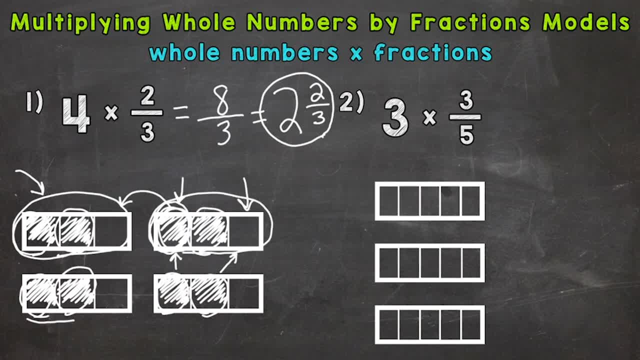 If we shifted some things around And then we're left with two-thirds here. So two and two-thirds. So our model matches that mixed number as well. It just takes a little bit of shifting around in order to make it work. So you can either go straight to that improper fraction and convert it to a mixed number. 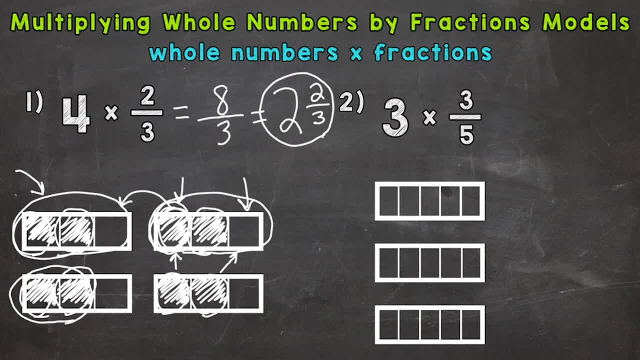 or shift things around and figure out what your mixed number is going to be. Either way. Either way, that model is going to give you the same and correct answer. So let's do number two, where we have three times three-fifths. 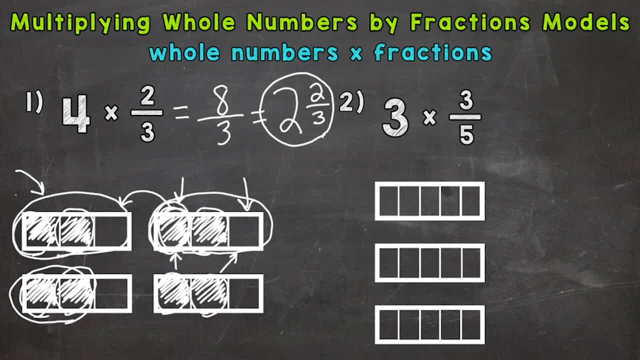 So we need three groups of three-fifths- And I already have our holes here- cut into fifths. So one-fifth, two-fifths, three-fifths, So that's one group of three-fifths- One-fifth, two-fifths, three-fifths. 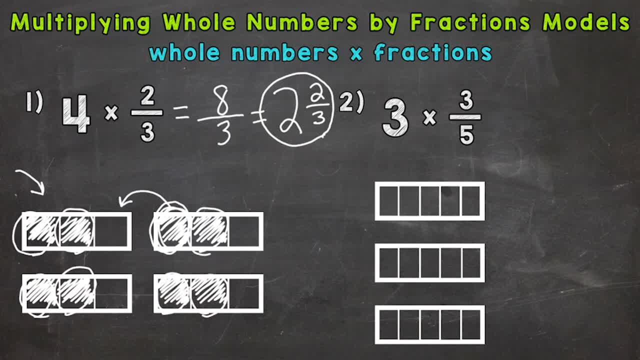 So that would make one hole there. if we filled that in, That would give us two openings: This one and right there. since we moved it, Let's move this to an opening and this to an opening, And that would give us Two holes filled in, right, if we shifted some things around. 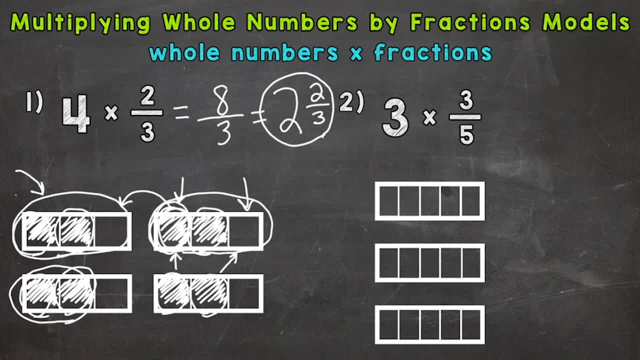 And then we're left with two-thirds here. So two and two-thirds. So our model matches that mixed number as well. It just takes a little bit of shifting around in order to make it work. So you can either go straight to that improper fraction and convert it to a mixed number. 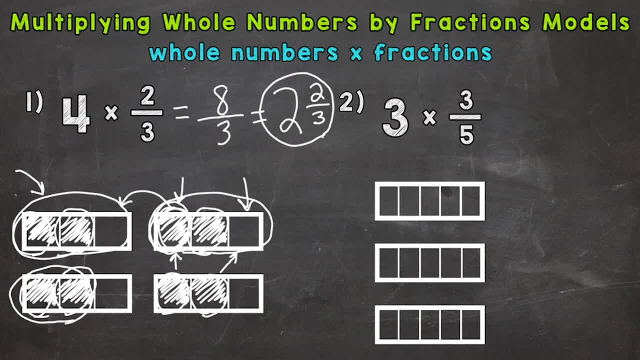 or shift things around and figure out what your mixed number is going to be. Either way, it's a good idea. Either way, that model is going to give you the same and correct answer. So let's do number two, where we have three times three-fifths. 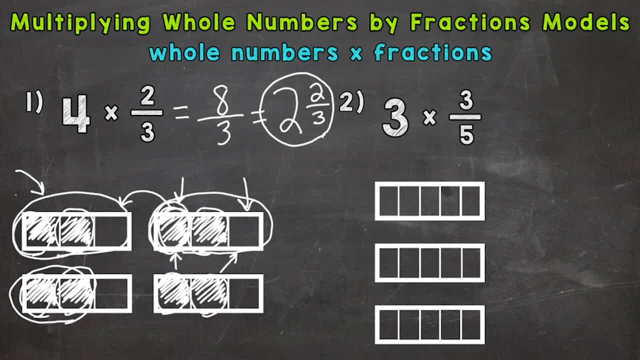 So we need three groups of three-fifths- And I already have our holes here- cut into fifths. So one-fifth, two-fifths, three-fifths, So that's one group of three-fifths- One-fifth, two-fifths, three-fifths. 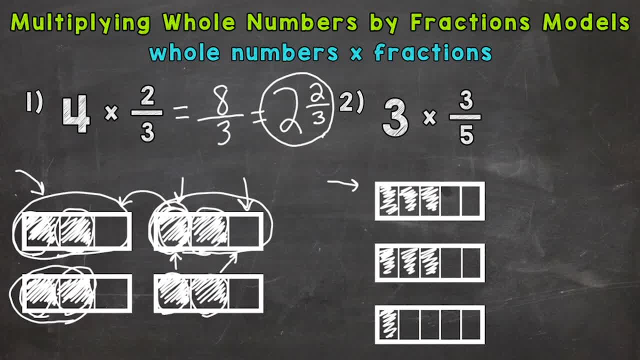 So we need one more group of three-fifths: One-fifth, two-fifths, three-fifths. So there we have three groups, or three times three-fifths. Let's see what our improper fraction is going to be. 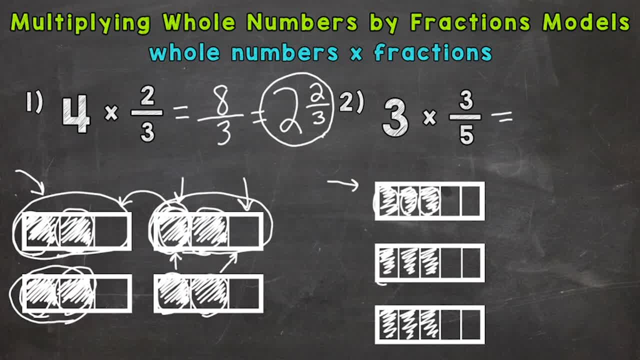 So one, two, three, four, five, six, seven, eight, nine-fifths, So nine-fifths. Now let's convert that to a mixed number. So how many, How many groups of five, whole groups of five can we pull out of nine? 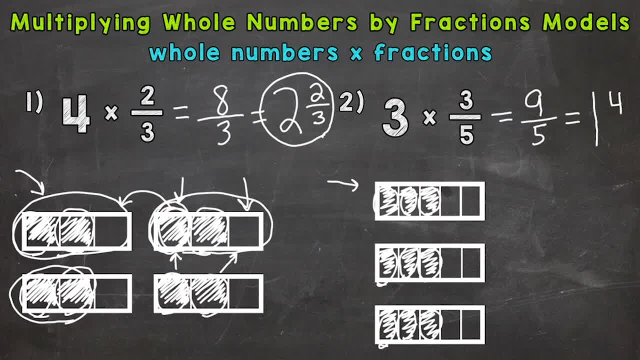 Well, one, And that gives us a remainder of four. Keep our denominator of five the same. So our answer is one and four-fifths. Now I'm also going to show you how to shift the pieces down in our model to equal one and four-fifths. 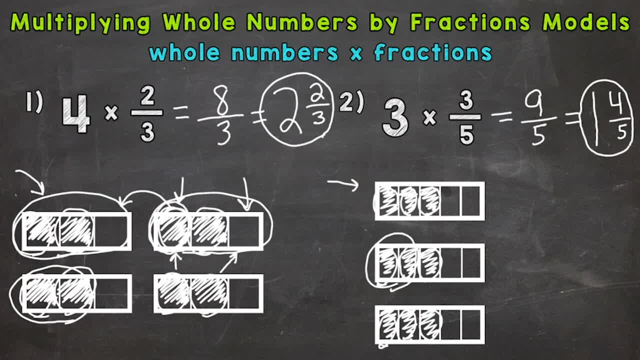 Let's take these two-fifths here and shift them up here, So we have one-fifth less. We have one-fifth left in that middle rectangle And we're going to take that one-fifth that is left and move it to the bottom rectangle. 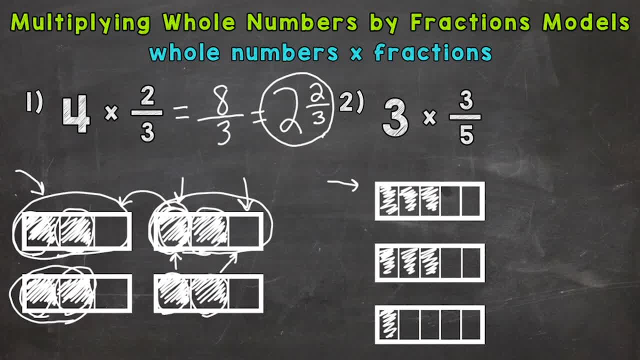 So we need one more group of three-fifths: One-fifth, two-fifths, three-fifths. So there we have three groups, or three times three-fifths. Let's see what our improper fraction is going to be. 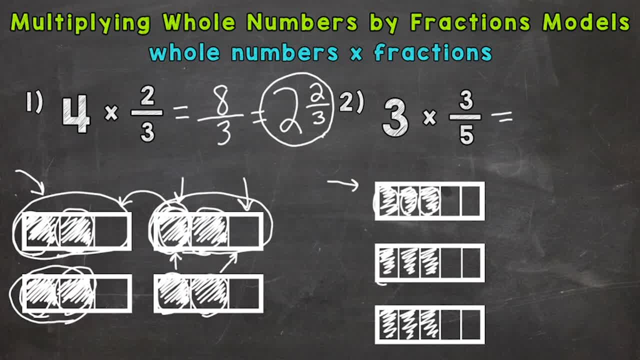 So one, two, three, four, five, six, seven, eight, nine-fifths, So nine-fifths. Now let's convert that to a mixed number. So how many, How many groups of five, whole groups of five can we pull out of nine? 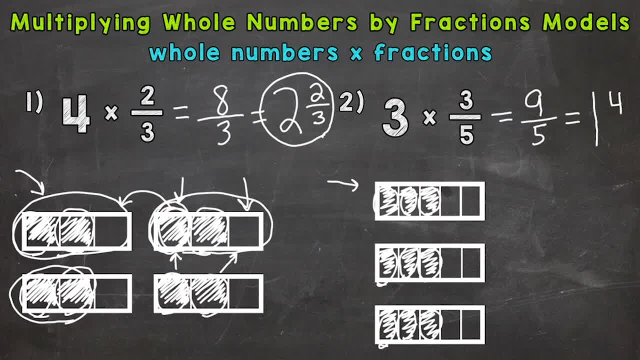 Well, one, And that gives us a remainder of four. Keep our denominator of five the same. So our answer is one and four-fifths. Now I'm also going to show you how to shift the pieces down in our model to equal one and four-fifths. 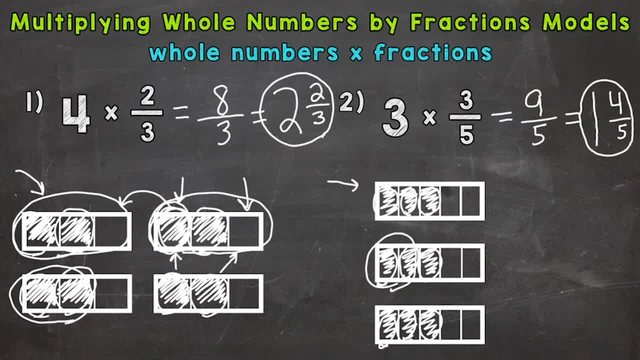 Let's take these two-fifths here and shift them up here, So we have one-fifth less. We have one-fifth left in that middle rectangle and we're going to take that one-fifth that is left and move it to the bottom rectangle. 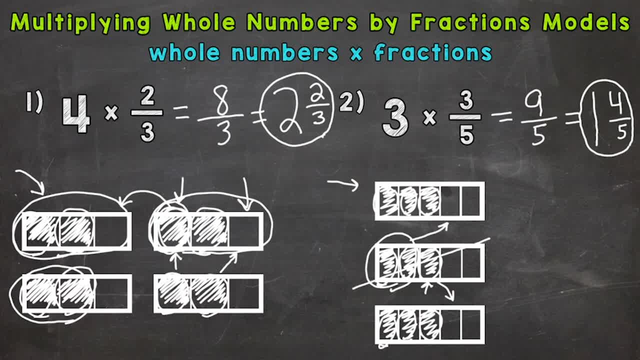 That way we get rid of everything. in that middle rectangle We took the two-fifths and moved them up to the top rectangle to make one whole. And we took that remaining fifth and moved it to the bottom rectangle in order to give us four-fifths. 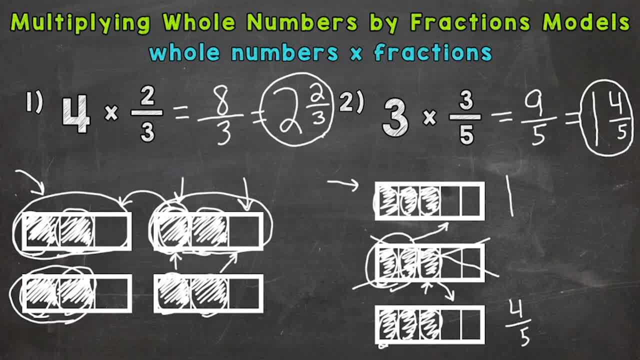 So after we shifted everything around, that model still matches the middle rectangle. So our answer is one and four-fifths. So there you have it. There's how you model multiplying whole numbers by fractions. I hope that helped. Thanks so much for watching. Until next time, peace. 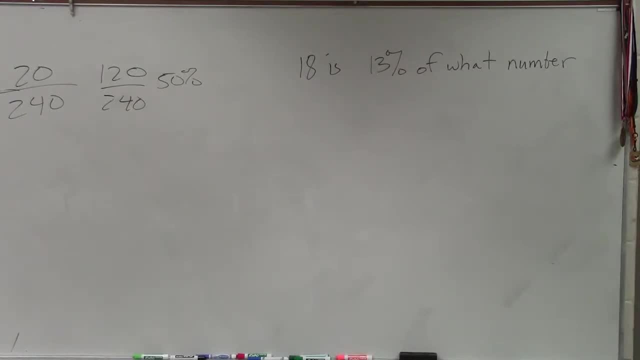 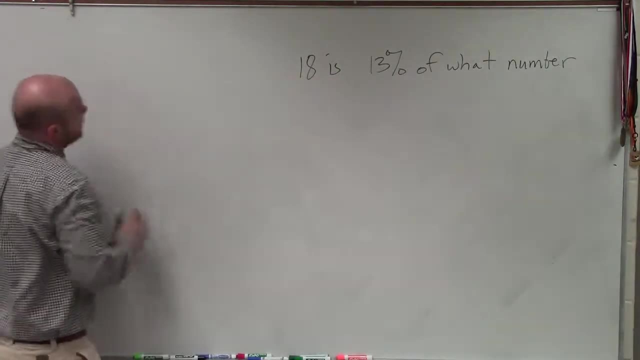 All right. So now on the next one, what we have here is 18, is 13%. of what number? So again, ladies and gentlemen, we need to go back Again, go back to well, all right, 13. What is our 13%? 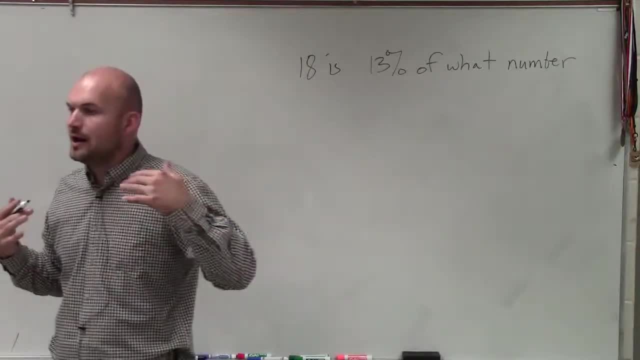 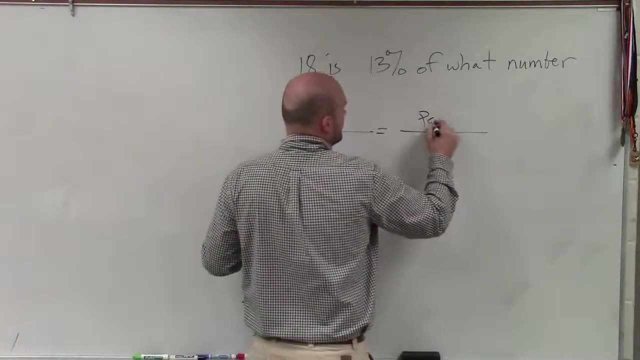 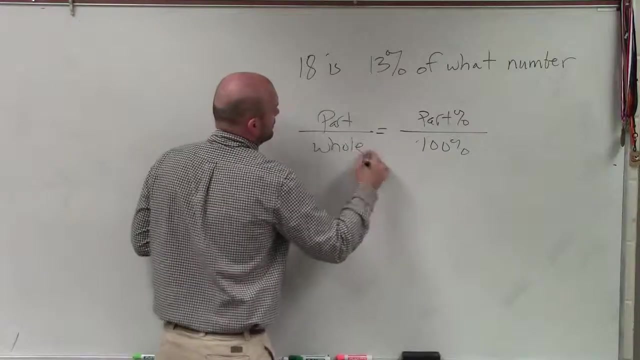 And again, guys, a lot of the time trying to rationalize and make sense of it, let's again just look at our proportion and just fill in what are the things we know: Part percent, 100%, 100%, part over whole. So if they're asking, if they tell us we have something, that's 13%.